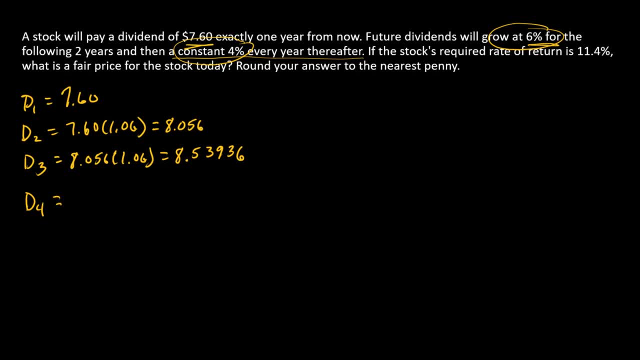 So I'll go ahead and write down D4.. D4 is 8.53936 multiplied by 1.04.. There's our lower growth rate. All right, so we know from this point forward that we've got a constant growth rate. 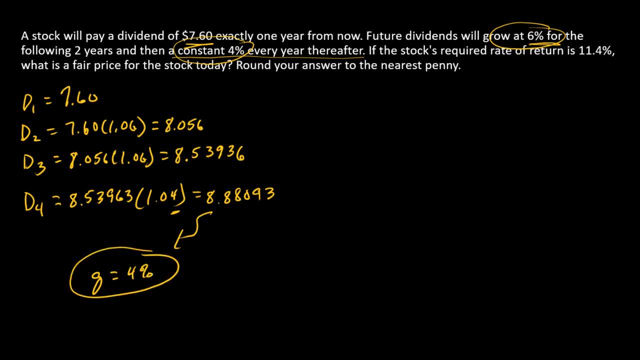 a 4% per year, a constant growth rate from year four onward, And so that's useful because we know, then, that the Gordon model is going to apply from time four forward, And so our price at time four is going to be something that we can calculate with the Gordon model. We know we need the next. 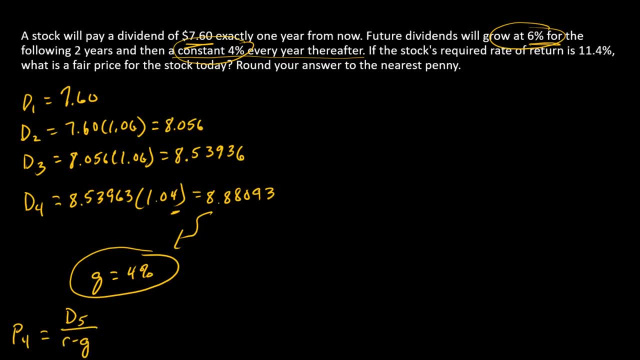 dividend in the numerator, R minus G in the denominator. So what's D5?? Well, D5 is the same thing as D4, grown at the long-term growth rate, And R minus G again is in the denominator. So inserting some numbers here, 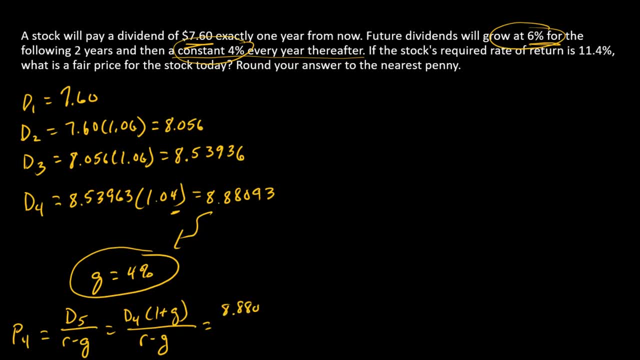 we have the following, And this gives us 124.8131.. So again, that's D4.. So what are we going to do with all this? We're going to go over and construct a timeline with four periods on it, So we can put D1,, D2,, D3, and D4 on the timeline, And then we can put P4 on the timeline as well. 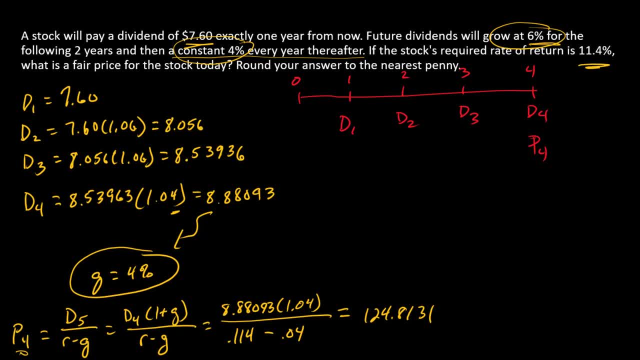 And once we do that, we can then, as a final step, discount each one of these back to the present, add them up and we have our estimate for the price. Okay, so let's go ahead and do that. So P0 is going to be the first dividend. So what's the first dividend? That's 760.. 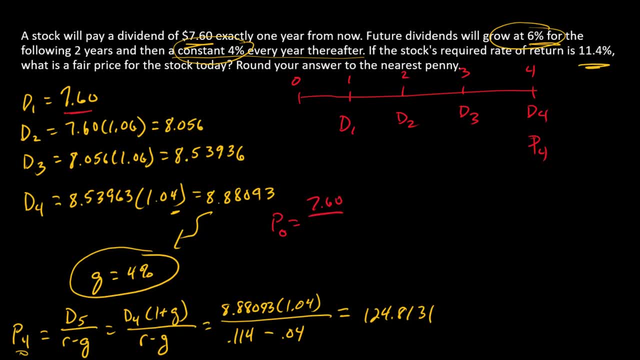 760.. That's going to be discounted one period plus the second dividend. So there's the second dividend And that's discounted two periods, And then we're going to have the third dividend. That'll be discounted three periods And then 6.60..